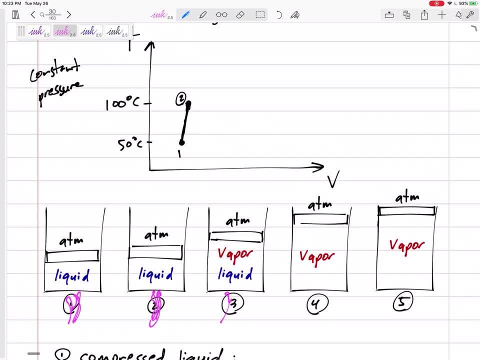 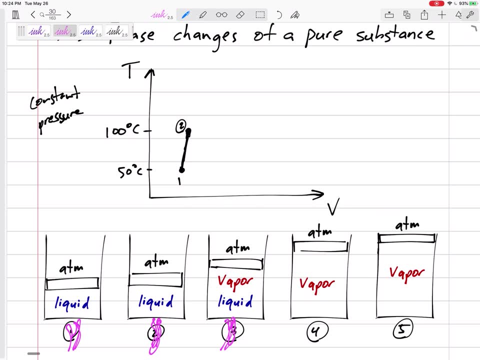 What happens? Do you know what happens when you put more and more heat to that? It starts vaporizing. right, It starts boiling, but the temperature- you all learned this in high school- right, The temperature stays the same. The temperature stays the same. 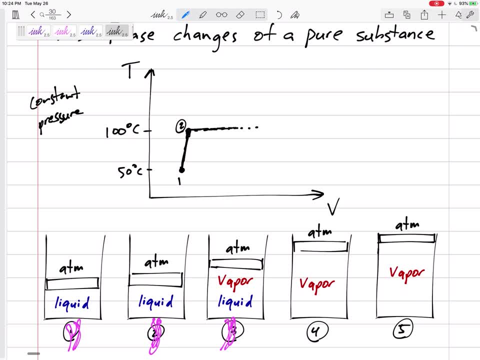 And so then we would go in this horizontal line and we'd get some liquid, some vapor, you know, and the volume would start to increase, but not much of a temperature change. And so then maybe we're at state 3, where there's a mixture. 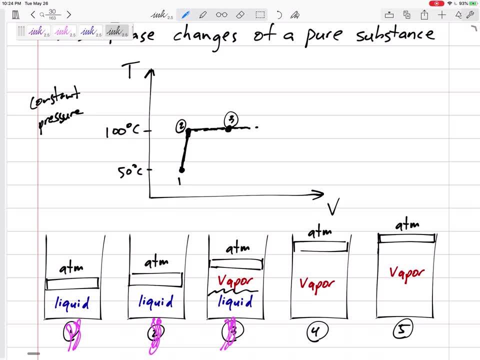 Some of the liquid is vaporizing, little by little or fast. you know Liquid Liquid is starting to vaporize And so maybe we've got half liquid, half vapor, A quarter liquid, three-fourths vapor. You know it is beginning to vaporize and the volume is increasing by a good bit. 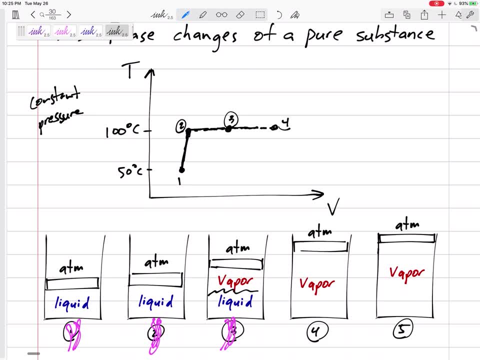 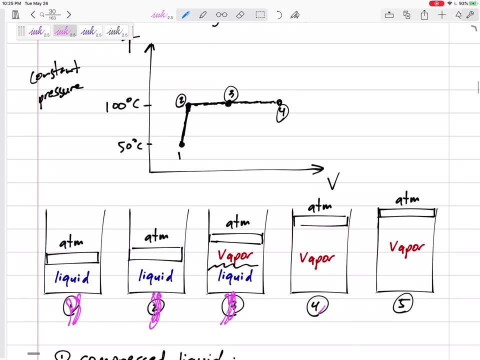 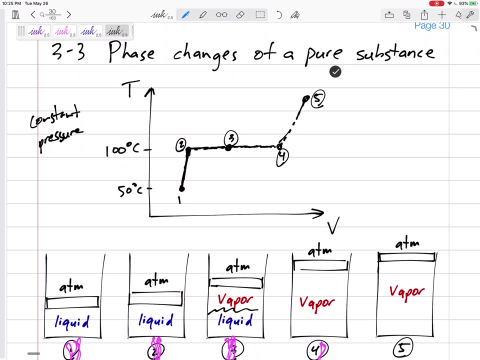 Alright. then it gets to a point where all of the liquid has vaporized. It gets to a point- we'll call it state 4, where all of the liquid has vaporized. And then what happens? if you add even more heat to it, then the temperature will start to increase. as it is all vapor now. it is increasing, its temperature is increasing, its volume is increasing. 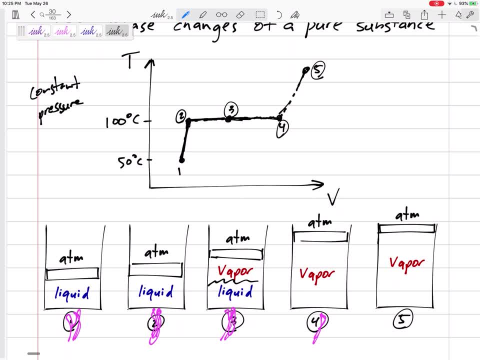 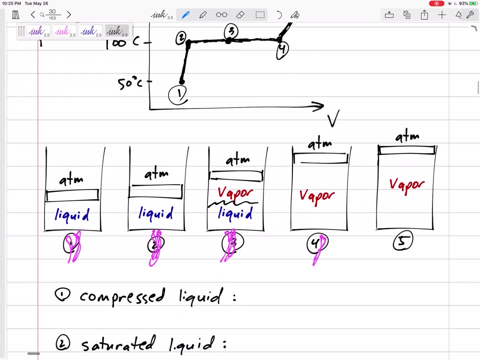 This is what a constant pressure phase change might look like. alright, And so it might go from state 1 to state 2 to state 3, to state 4 to state 5.. So let's look at each of these. These are kind of interesting points on the phase change graph. 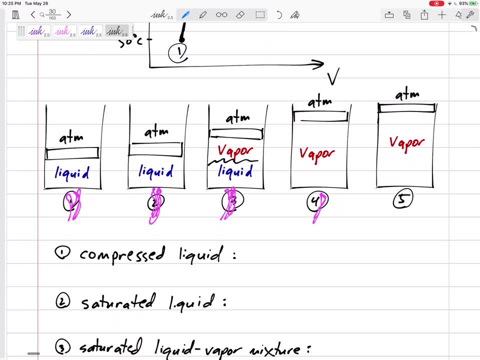 Alright, state 1, is a compressed liquid. Alright, it is 100% liquid. Alright. it's also known as a sub-cooled liquid. Alright- most all liquid water that we think. we think of water. it's a compressed liquid. 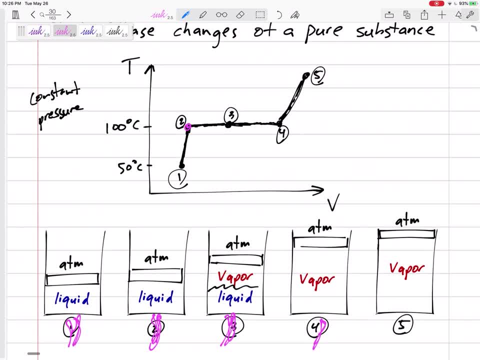 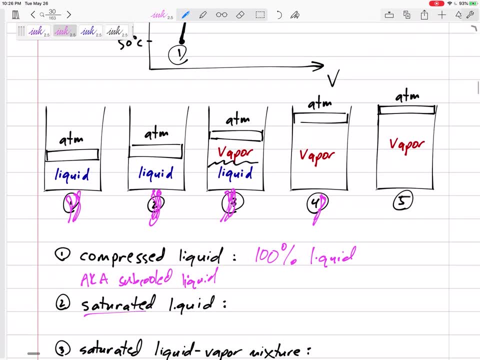 Alright. but then it gets to point 2, which is the point at which it just begins to vaporize. Alright, and so that is, we're calling it a saturated liquid. That is saturated liquid. It is still 100% liquid. 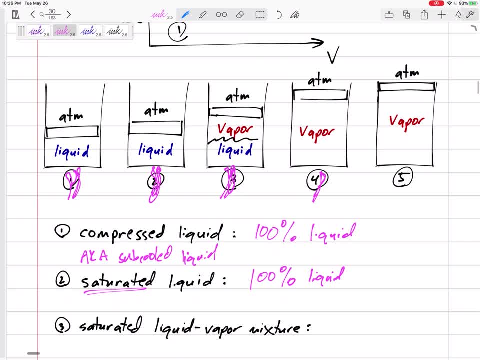 Right, it is still 100% liquid, but it is just beginning to vaporize. It is about to vaporize. Any infinitesimally small increase in heat and it would start to vaporize, But at a saturated liquid it is still 100% liquid. but that's the last point, that it's 100% liquid. 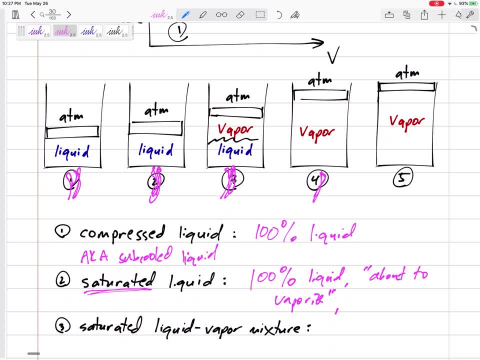 Anything above that and it is going to be a mixture. So it is 100% liquid, it's about to vaporize and it is at the saturation temperature. We think of it as the boiling point or the boiling temperature. But this It's saturation temperature is the temperature at the phase change. Saturation temperature is the temperature of the phase change. Okay, Alright, then at state 3, it's a saturated liquid, saturated vapor mixture, Alright, So it's not like all of this liquid. 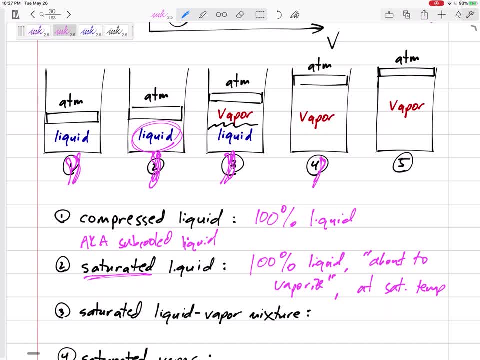 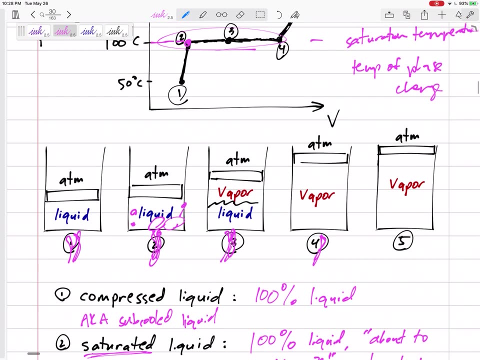 All of it changes slowly to vapor. It's a portion of liquid goes straight to vapor, Another portion of liquid, you know, another particle goes straight. All of these particles are going straight from liquid to vapor. So So it's a mixture, right? 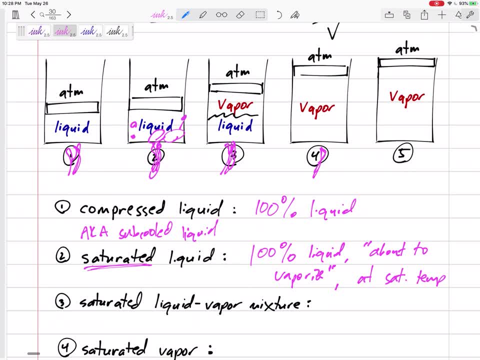 It's a mixture. A little bit of it has changed, A little bit more of it has changed, A little bit more of it has changed, A little bit more of it has changed, And so it's a saturated liquid vapor mixture. 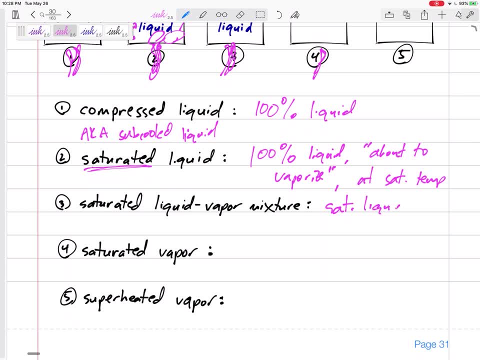 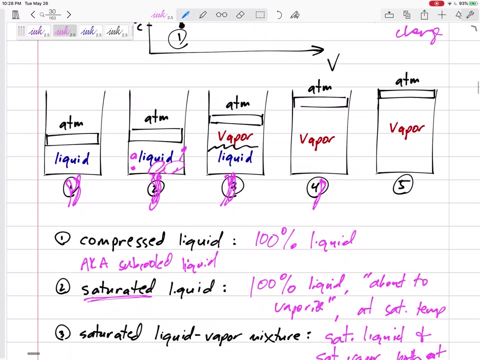 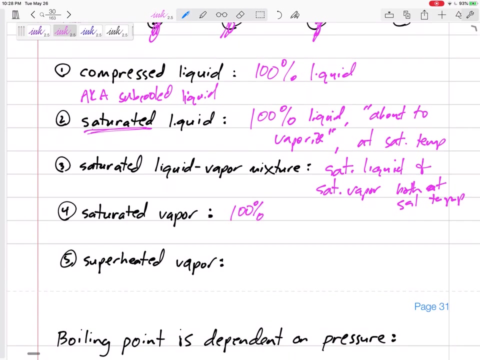 It is saturated liquid and saturated vapor. Both of them are at the saturation temperature. Saturated liquid and saturated vapor, both are at the saturated temperature, Alright. And then when it gets to point 4. Which is still at saturation temperature, But it has all 100% converted to gas. 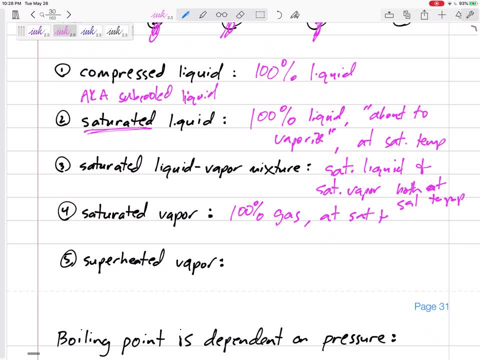 It is at the saturation temperature. It is on the verge of going back of condensation. Any decrease in heat If you let off any on that heat, It's going back to Back to a mixture, Back to a mixture, Alright. 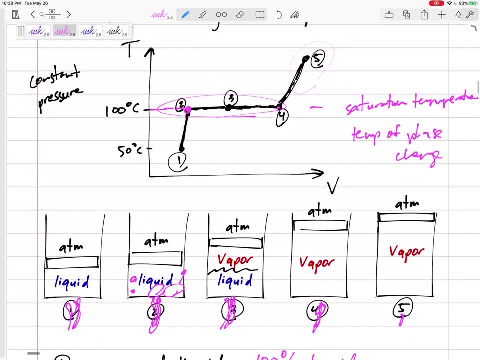 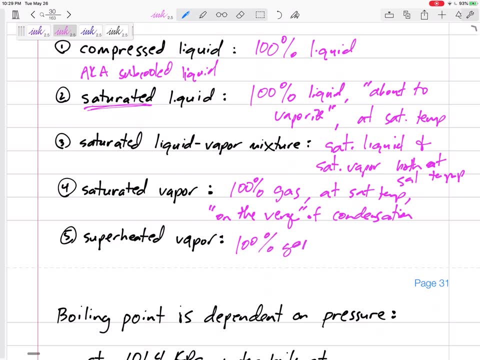 And then if you add even more heat And we get out here anywhere past point 4. Then it's a superheated vapor, It is 100% gas, 100% vapor. And now the temperature has risen. It is above the saturation temperature. 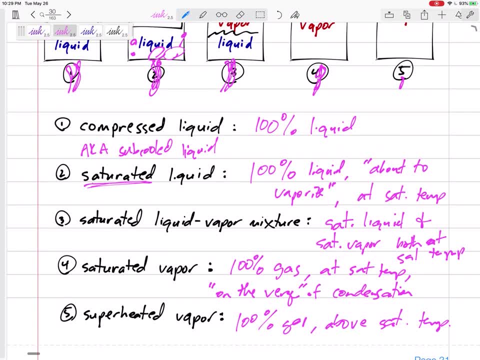 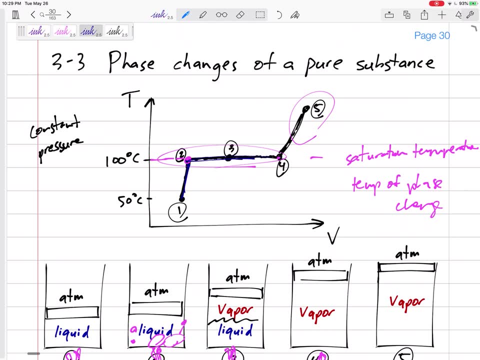 It is above the saturation temperature. Okay, That was one example. This is at one pressure. Maybe atmospheric pressure right here, At a different pressure, it would have a different line. Maybe it's right here At a different pressure, it will have a different constant pressure line. 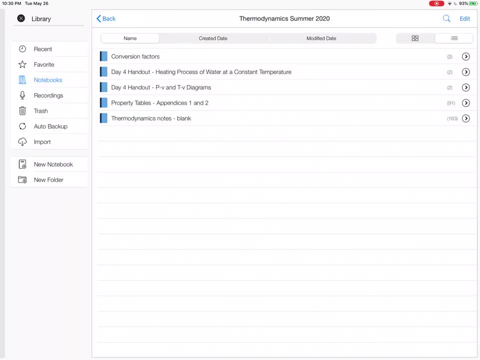 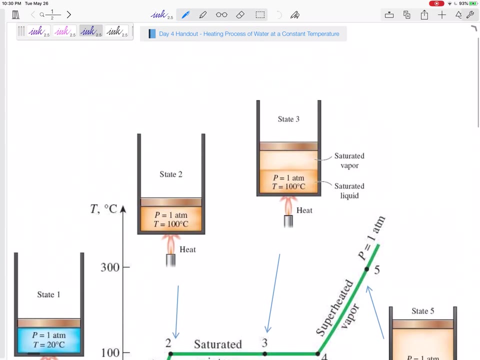 Alright, So that's a good page, But let's go to our handout right here. Yes, And so I took the figure in the book And tried to edit it to visualize it, And so this is what we were doing. This is what we were doing. 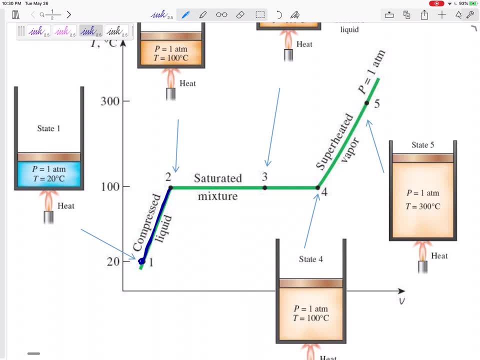 We start right here. We add some heat, It gets to the saturation temperature And then it starts. Some of it: A little bit of liquid changes to vapor. A little bit of liquid changes to vapor. A little bit of liquid changes to vapor. 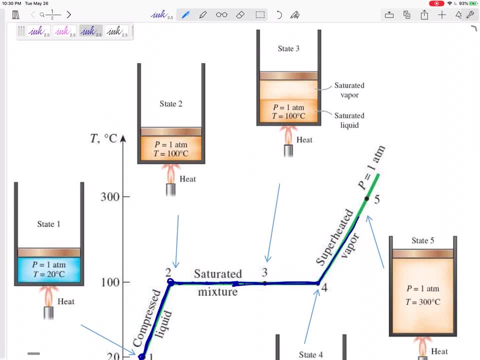 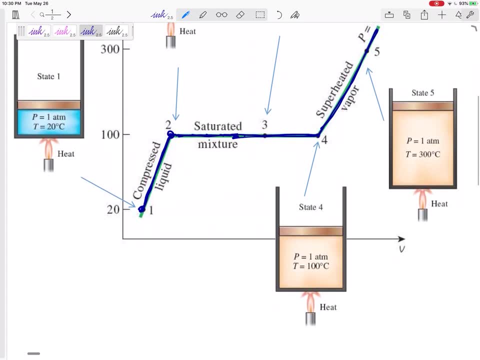 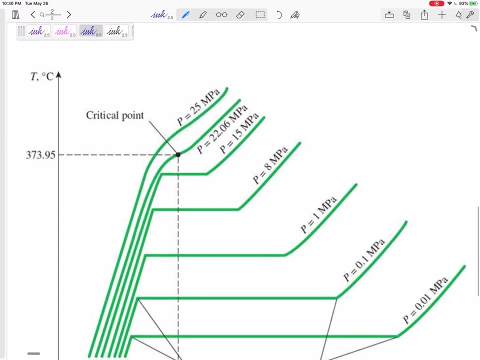 From 2,, 3,, 4.. And then we have a superheated vapor anywhere above 4.. Okay, So this is a constant pressure phase change. right here A TV diagram of water at constant pressure, Now at different pressures. 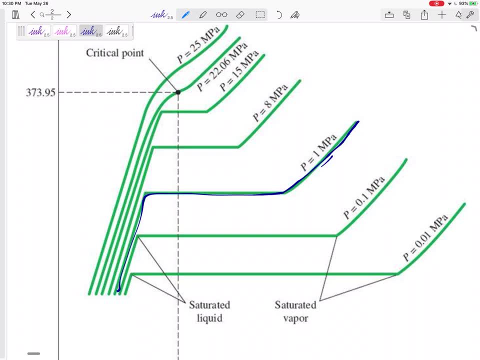 At different pressures. then we have different lines. So this is at 1 MPa, This would be at 8 MPa, This would be at 15 MPa. So different pressures have different saturation temperatures. This pressure right here Would have: 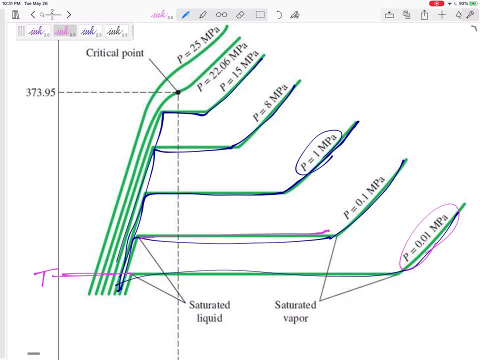 That saturation temperature. This pressure right here Would have that saturation temperature. This pressure would have that saturation temperature. This pressure would have that saturation temperature. Did you know that if you're boiling at a very high Elevation, right Above sea level? 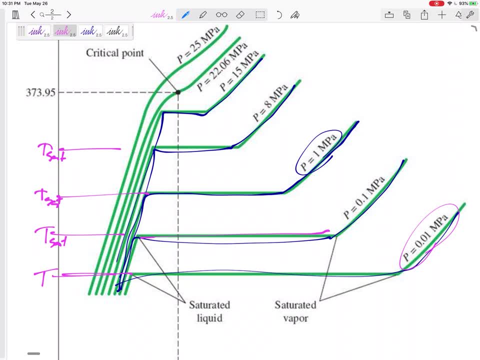 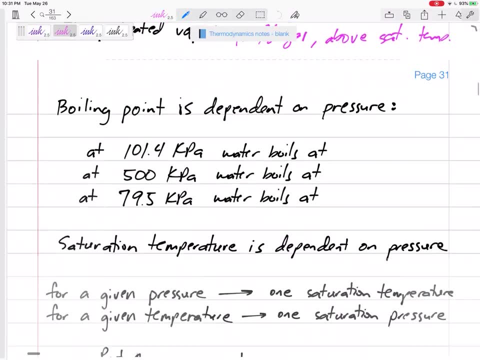 Where the pressure is different, right Where the pressure is lower, Your water will boil at a different temperature. Let's go back to our Let's go back to our notes. Let's go back to our notes. Did you know that boiling point is dependent on pressure? 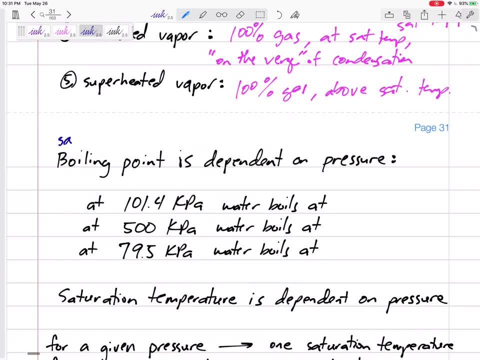 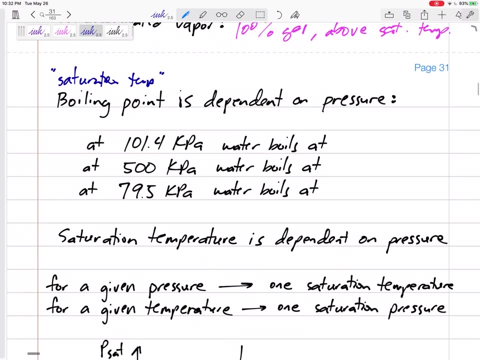 And we're saying boiling point, because I think of boiling of water, But also we're talking about saturation. temperature is dependent on pressure. We just showed that with all those different pressures, with different lines At about atmospheric pressure, water boils at 100 degrees Celsius. 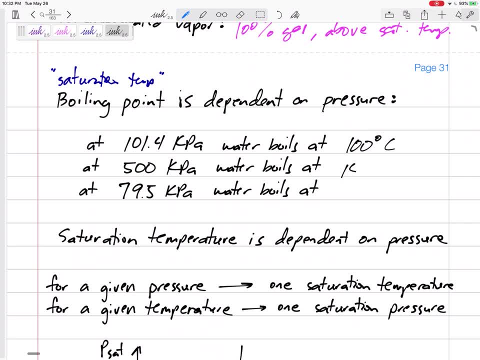 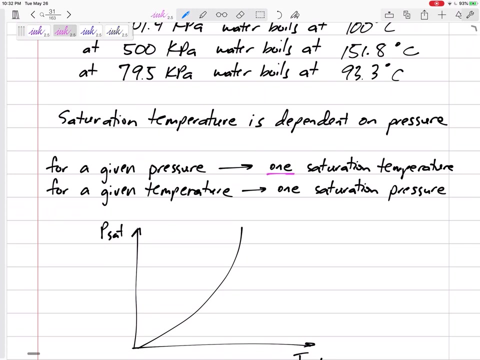 But if the pressure was higher it would take 151.8 degrees Celsius to boil water. If the pressure is lower, water boils at 93.3 degrees Celsius. Saturation temperature is dependent on pressure, But for a given pressure there is only one saturation temperature. 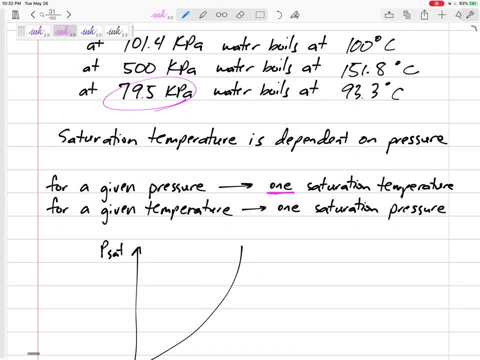 Alright At For that. It's material, You know. for that, pure substance: Alright. So water at this pressure, it will boil at 100 degrees C. Alright For water. You know, water at this pressure boils right here. 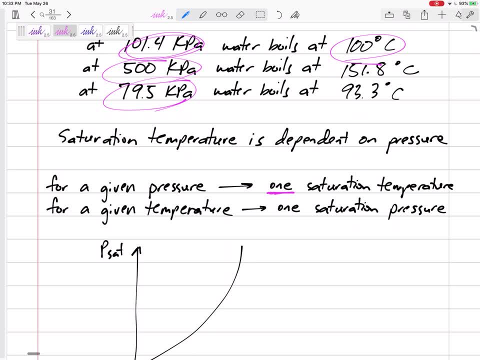 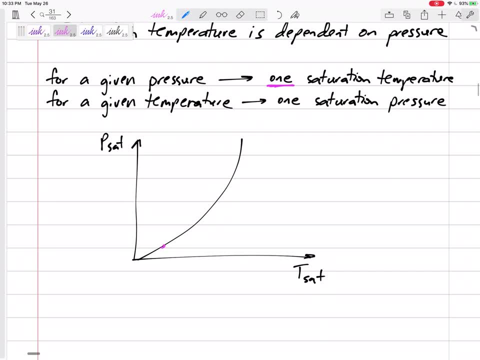 It's a one-to-one. For a given pressure, there's one saturation temperature. For a given temperature, there's one saturation pressure. There's one pressure that this phase change happens, And it's maybe this line right here For this temperature. 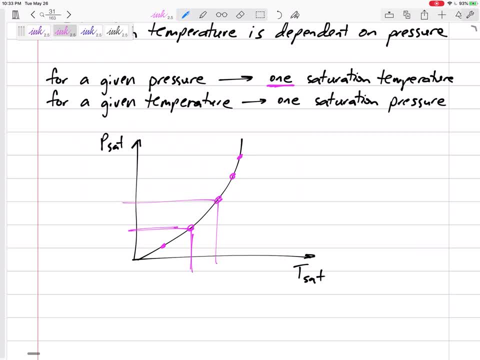 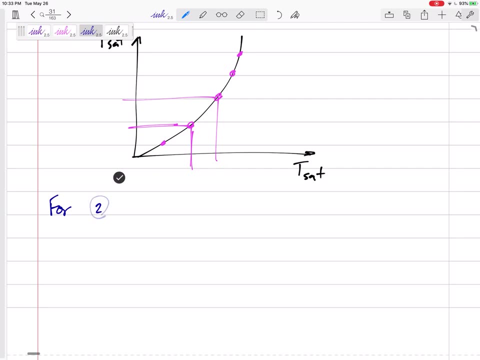 That's the pressure For this temperature. that's the pressure. It's not like there's two different temperatures and pressures. Okay So, because there's kind of this one-to-one thing, then if I am at point two, if I'm a saturated liquid, 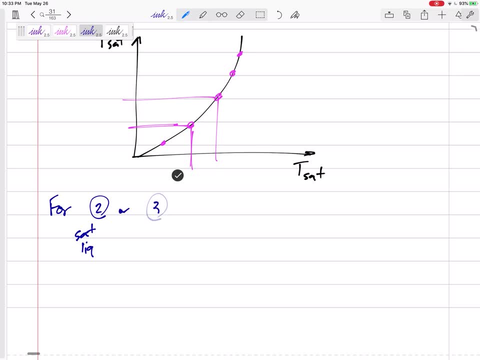 or if I'm a mixture, a saturated liquid-vapor mixture, or if I'm a Saturated vapor anywhere on two, three, four, then they are at the saturation temperature and pressure. So I know these are at saturation, the saturation point. 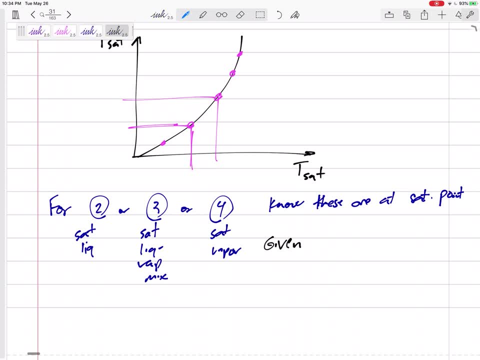 So here we go. So if you are given the temperature- and I'm at point two, three, four- if you are given the temperature, then I know the pressure. I don't need any other information. You know if I know it's water. 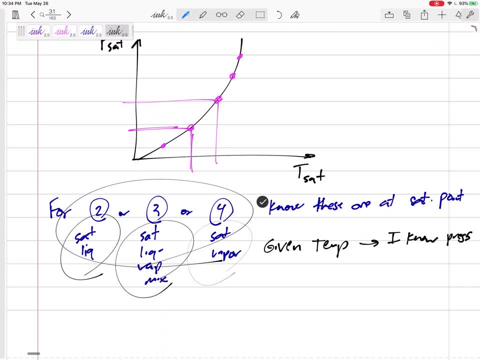 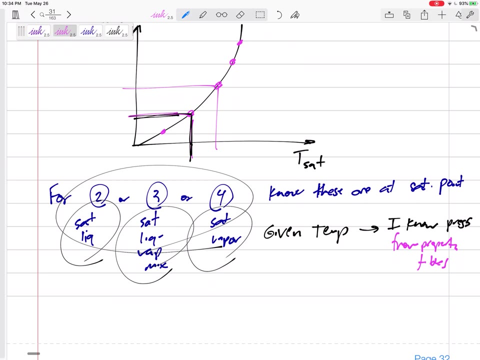 and I know the temperature and I know it is either a saturated liquid, saturated vapor or a saturated liquid-vapor mixture. then from the property table I can get the pressure. From property tables I can get the pressure. Same thing. 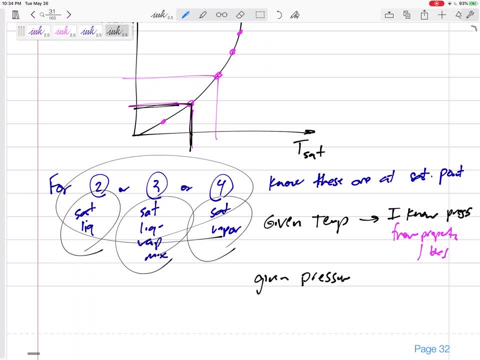 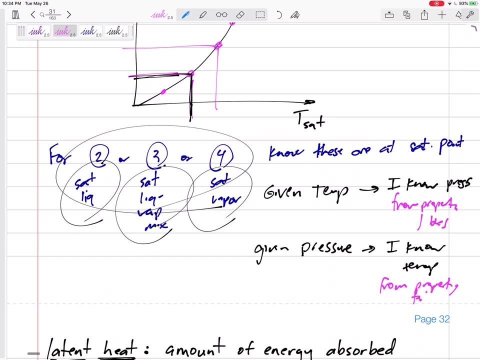 If we are given the pressure- and I know it's at state two, three or four- then we can get the temperature from property tables. These are the property tables that are in the back of the book. We'll talk about these. 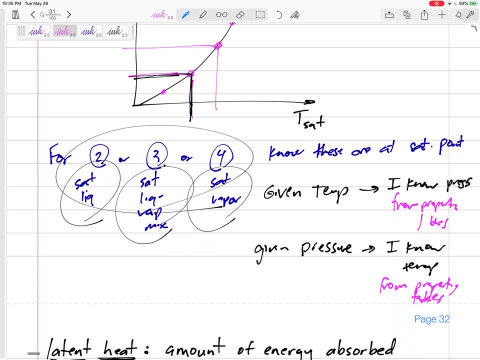 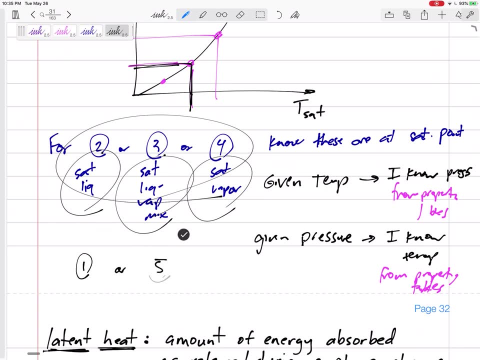 These are property tables that you will have printed out already when you get into the test. But state one or five, then no. If you tell me the temperature, I'm going to need some more information- All right, Whereas if I'm at state two, three or four, 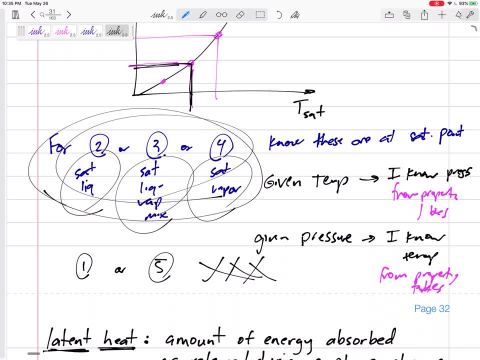 you tell me the temperature and then I can look: okay, what is the saturation pressure for that temperature. Or you give me the pressure. I say: okay, what is the saturation pressure for that temperature, If I may have said that backwards. 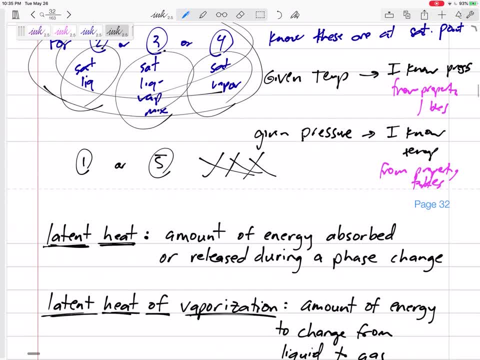 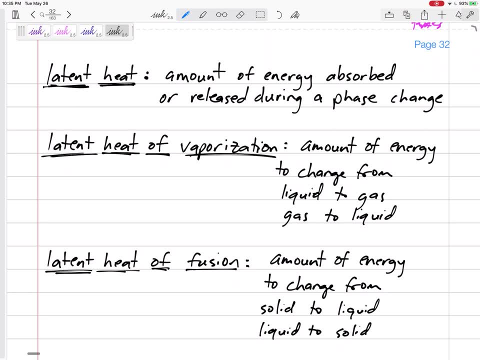 Okay, All right, We'll talk about the property tables in just a minute. One more page of just kind of some definitions. Latent heat is the amount of energy during a phase change. All right, The amount of energy required for a phase change. 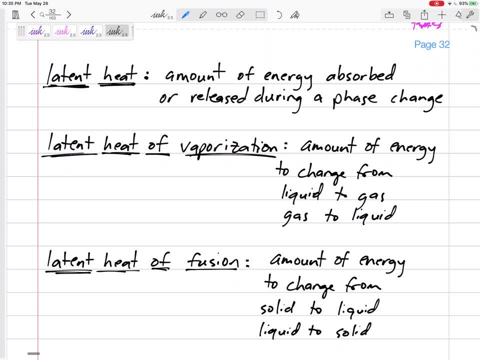 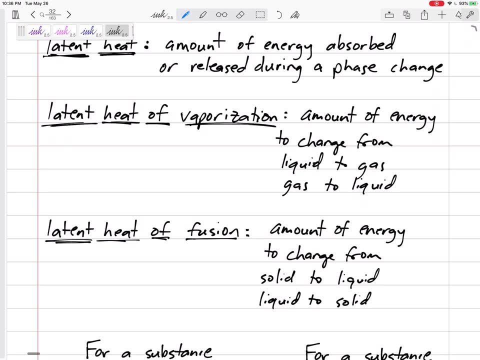 or the amount of energy released during a phase change, whether it is vaporizing or fusion or condensing. All right, So the latent heat of vaporization is the amount of energy or the amount of heat to change from liquid to gas or gas to liquid. 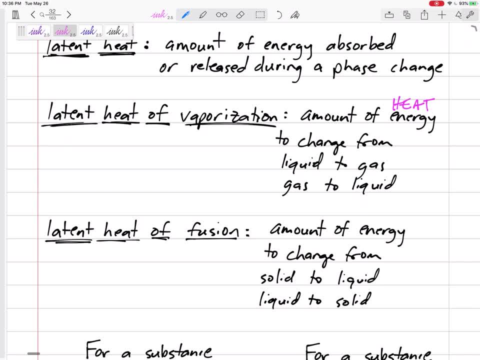 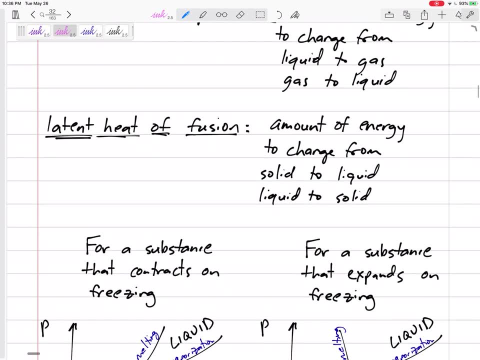 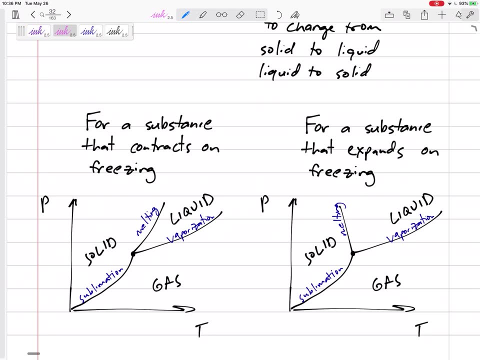 to change completely from liquid to gas or gas to liquid. That's the latent heat of vaporization. The latent heat of fusion is the amount of energy to change from solids to liquids. Solids to liquids: All right For a substance that contracts on freezing. 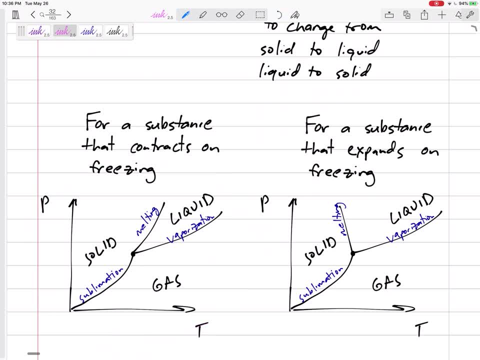 this is kind of its phase diagram. So for probably atmospheric pressure, most substances right at a low temperature will be solids, and then here they'll be liquids and then they will be gases At very low pressures, though sometimes things can. 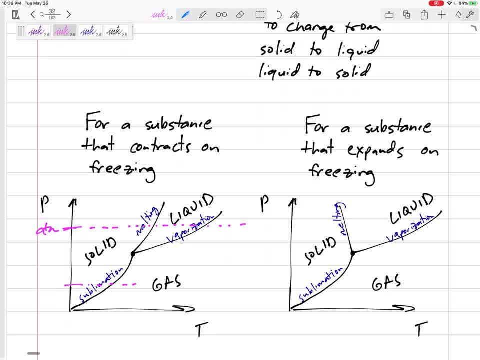 it depends on the substance, at what pressures these happen, but sometimes things can go straight from solids to gases. All right, Straight from solids to gases. For substances that expand on freezing, their phase diagrams look a little bit more like this, where we've got this right here. 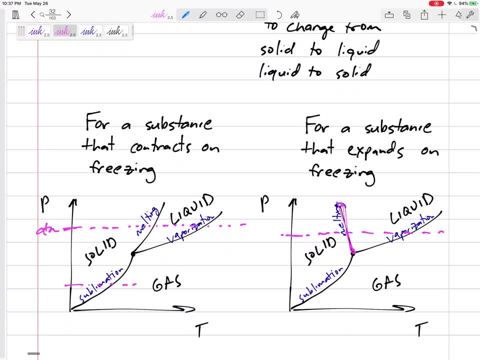 where that melting line goes in this direction to the left. So larger pressures, you actually have a smaller, a less temperature needed to change from solids to liquids. Right there, All right, Water is water is a phase diagram looks like that. 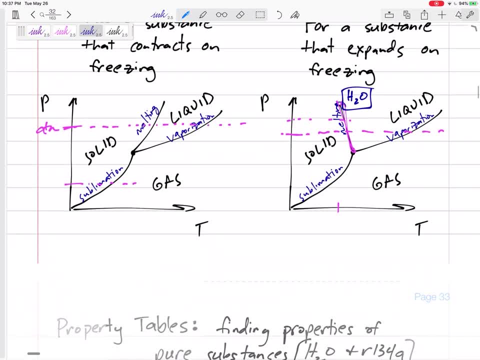 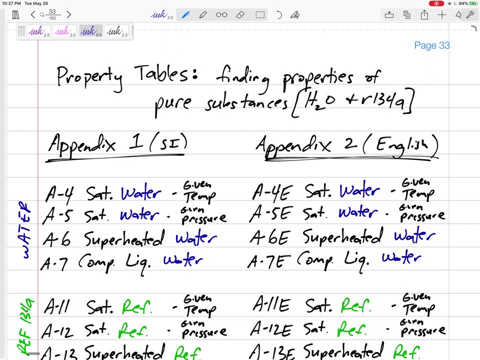 right there. Okay, Let's talk about these property tables. So we're we haven't used them yet. This is our first, our first look at our property tables, So let's get comfortable with them. Here are our property tables. 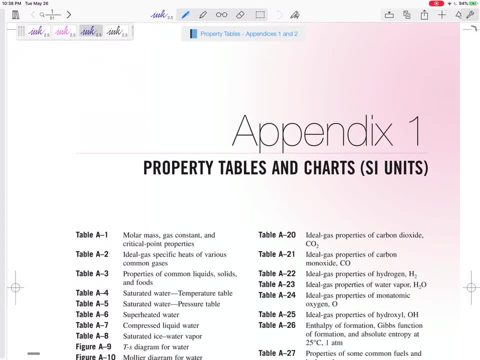 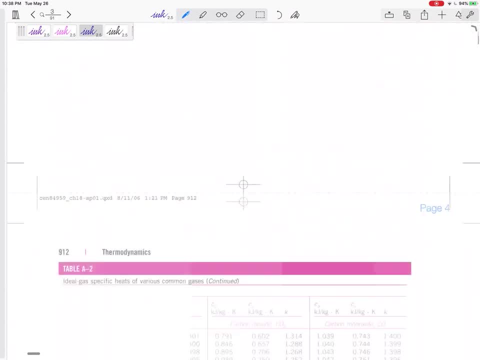 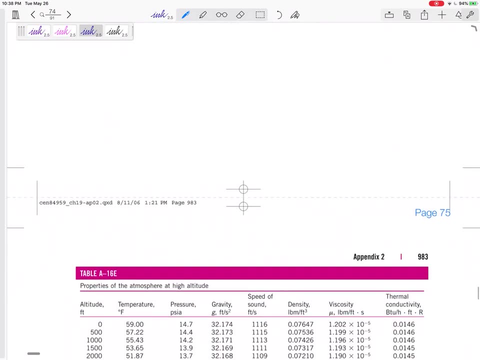 Appendix one and appendix two in the back of our book. Appendix one is SI units. Appendix two is English units. All right, So appendix one is SI units. It's a lot of pages, right, 40, 50 pages. Appendix two: 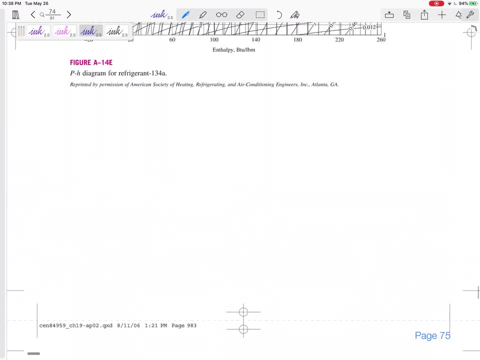 it is. it has an E on all of these. They're the English units And you can look at the units. You know you'll see lots of English units, SI units on appendix one. So here's a kind of an overview. 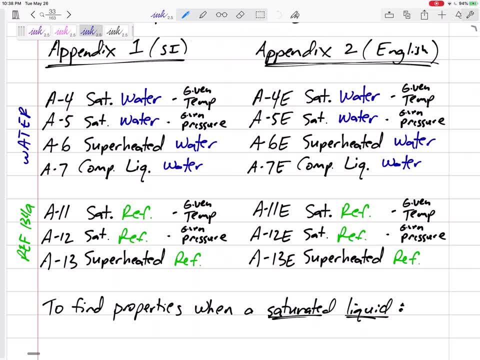 of the property tables that we need to be looking at right now. All right, Let's look at four, five, six, seven and 11, 12, 13.. All right, Four, five, six, seven and 11, 12, 13.. 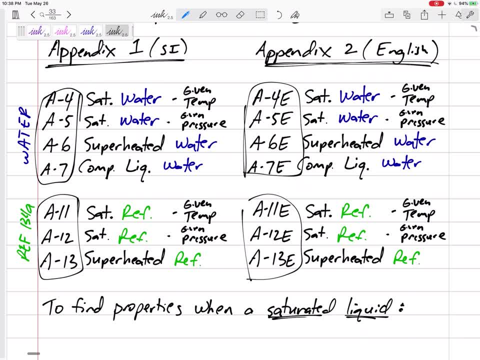 So let's forget about everything else. Don't get bogged down in one, two, three and eight, nine, 10, and all the higher ones, Because we're looking at pure substances, All right, So do you see that? four, five and six. 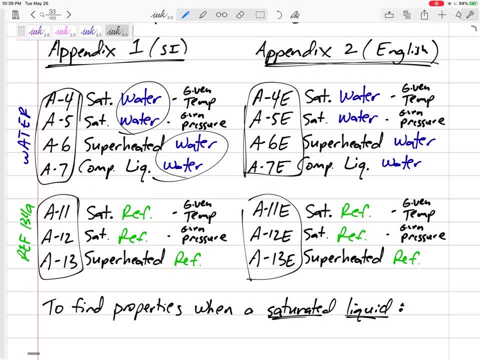 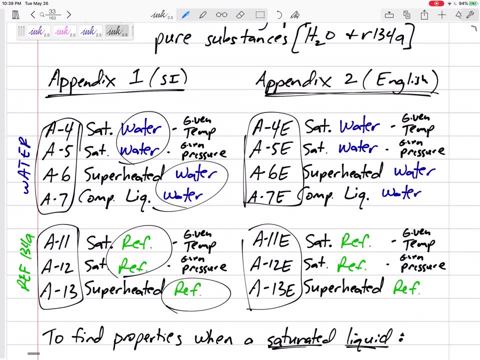 are for water. Four, five and six are for water, Whereas 11,, 12,, 13 are for refrigerant. All right. Refrigerant, a different pure substance, Refrigerant 134A. All right. So appendix one is SI units. 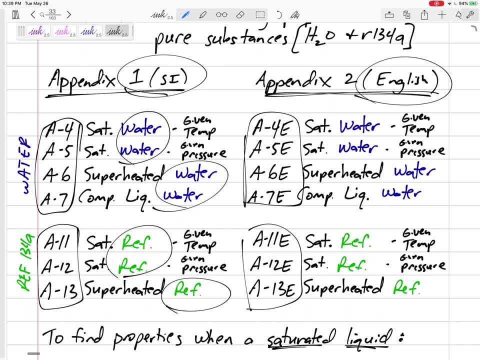 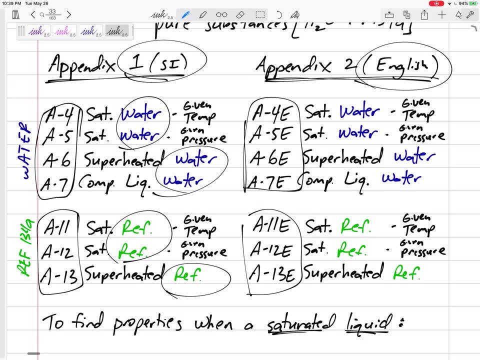 Appendix two is English units. So that's kind of the first thing. Is my problem in SI units or is my problem in English units? Okay, Then the next thing is: am I talking about water and am I talking about refrigerant? If I'm talking about water, 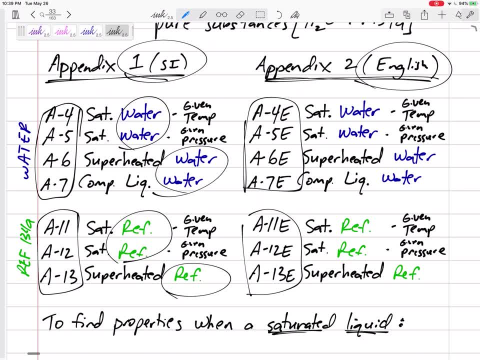 then I'm looking at tables four, five, six, seven. If I'm talking about refrigerant, I'm looking at tables 11,, 12, 13.. Okay, Four and five are saturated tables. Okay, Four and five are saturated tables. 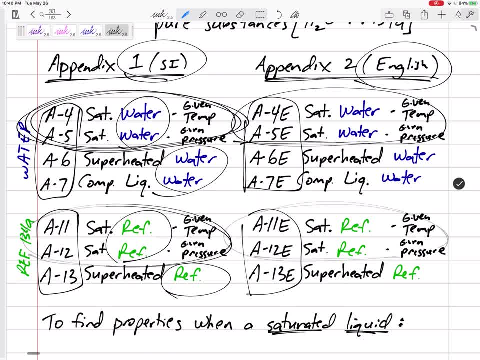 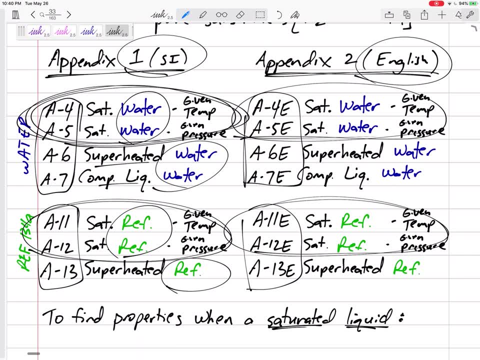 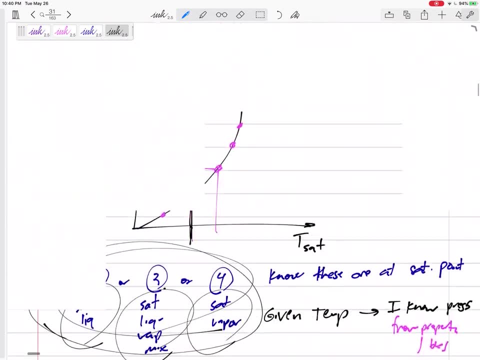 Or 11 and 12 are the saturated tables. 11 and 12 are the saturated tables. Six is superheated, Seven is a compressed liquid. right Six is superheated. Seven is a compressed liquid. So if we're kind of going back to this right here, 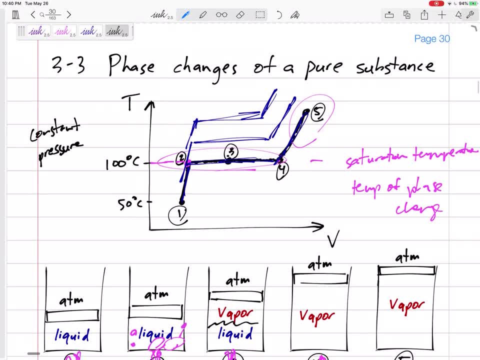 this: one, two, three, four, five, Two, three and four. I would be at the saturation temperature: Two, three and four. I would be looking at the saturated tables, Tables four and five or 11 and 12.. 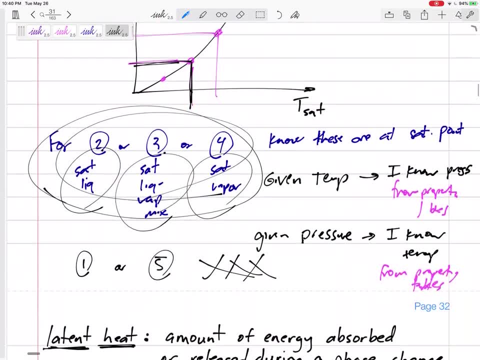 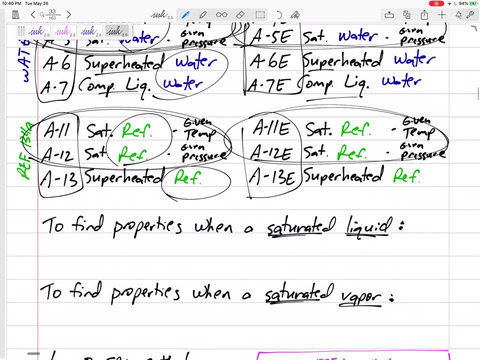 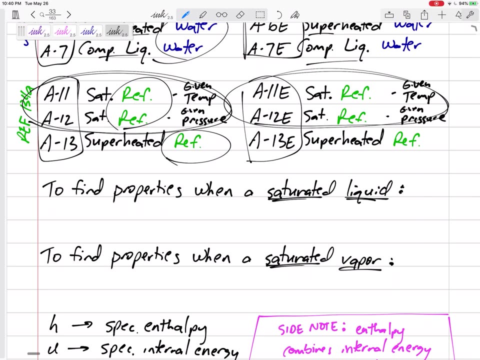 Okay, Whereas if I'm superheated, I would look at the superheated table, If I'm compressed liquid, I would look at the compressed liquid tables. Okay. So let's start with points two and four: a saturated liquid and a saturated vapor. 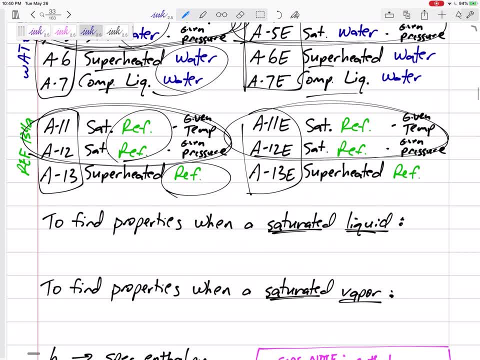 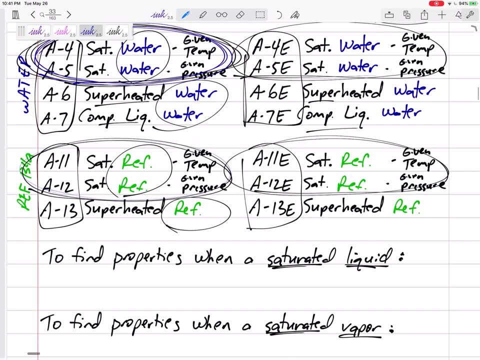 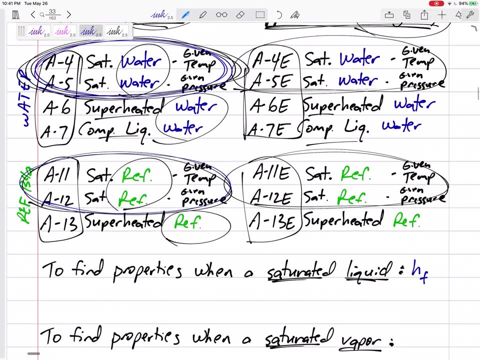 To find the properties of a saturated liquid or a saturated vapor, I would go to the saturation tables four and five or 11 and 12.. The saturated liquid properties have a subscript F, So H F U. subscript F. 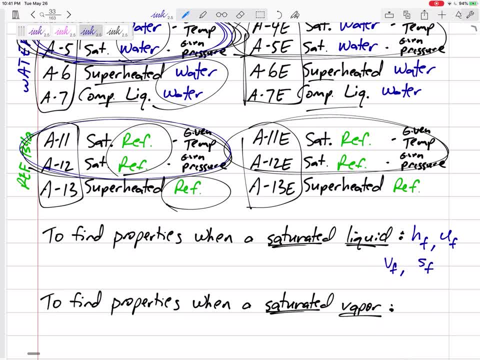 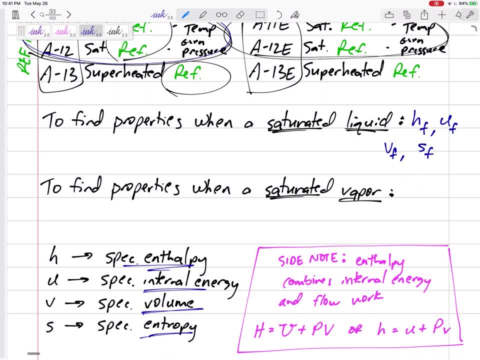 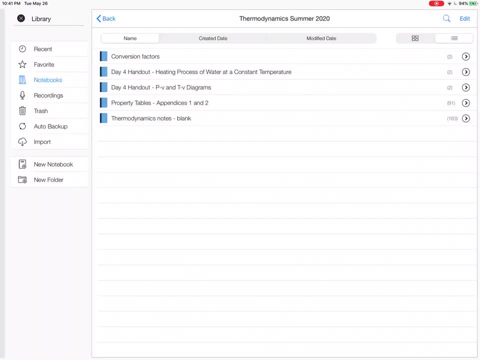 V, subscript F. S subscript F: All right, H is enthalpy, U is internal energy volume and entropy. So anyway, the saturated liquid properties have subscripts F. So let's go to tables four and five. I went way too far here. 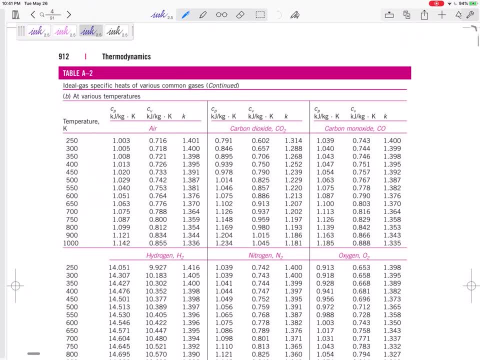 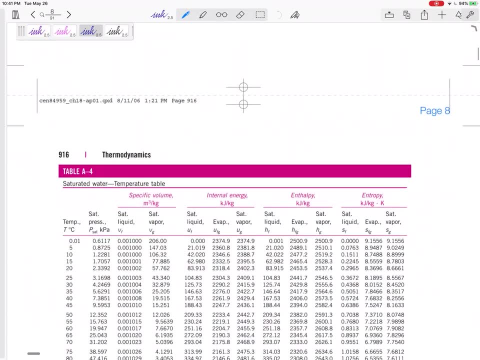 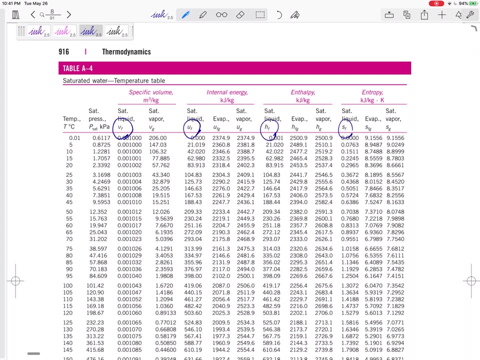 Let's go to tables. all right, three is we're not worried about we need to get to. that's table A2, table A3, table A3. here, table A4.. All right, So here. VF, UF, HF, SF. 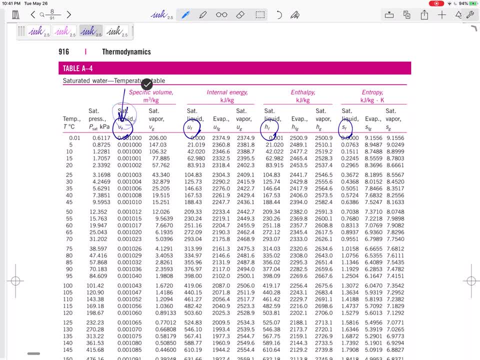 that is the saturated. if it is, and it tells you right here, it is a saturated liquid. So maybe I know it's a saturated liquid at that temperature. There's its specific volume, Here's its internal energy, Here's its enthalpy. 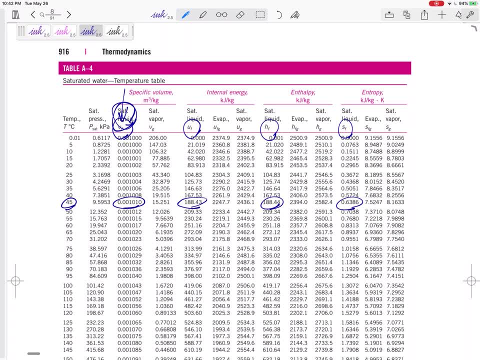 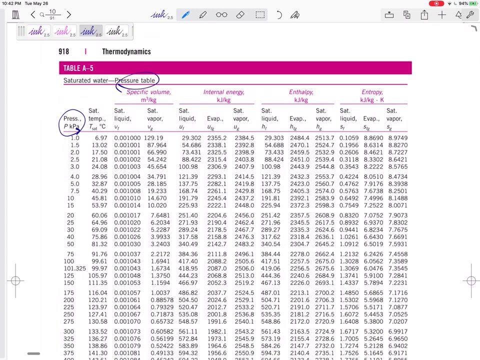 Here's its entropy. So the subscript F are the saturated liquid properties. All right. Table A4 is for water. It is saturated and it is organized by temperature, Okay, Whereas table A5 is organized by pressure. So if we know it is saturated liquid. 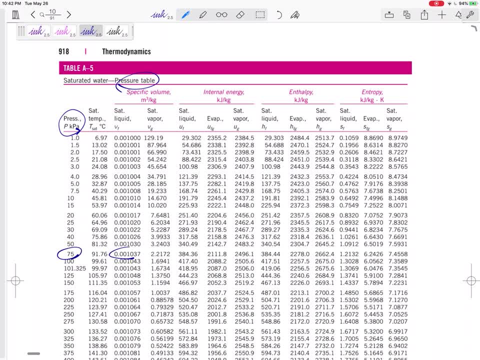 and we are given the pressure. then we would come to the pressure table and any of these subscript F are the saturated liquid properties. All right, Saturated, that's the easiest one. Saturated liquid properties are these on the subscript F, column right here. 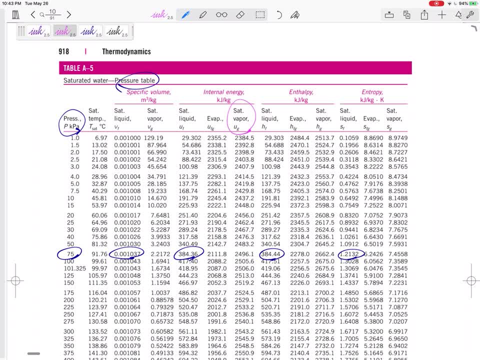 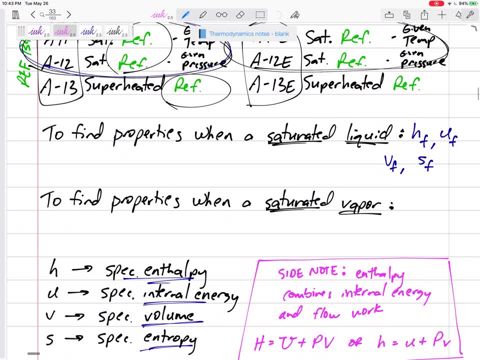 Well, what do you think saturated vapor properties are? They're these right here, right? Subscript G, Subscript G. So let's go back to our notes. This would be HGU, subscript GVGSG. Those are the easiest. 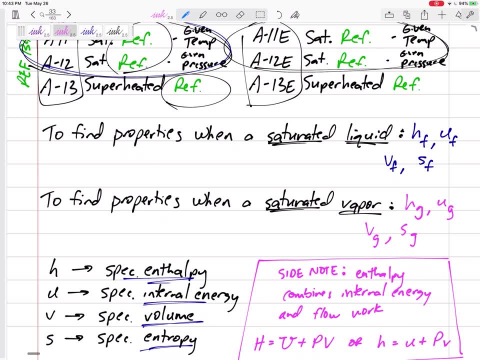 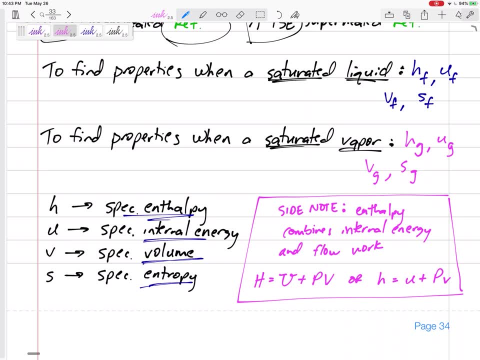 That's what we're going to start with: Finding the properties if it's a saturated liquid or if it's a saturated vapor. So H is enthalpy. We haven't talked about enthalpy. Enthalpy, briefly here, combines internal energy and flow work. 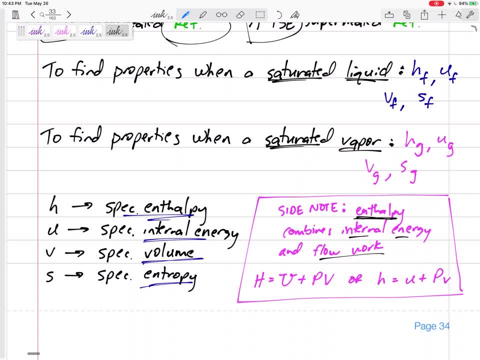 All right. So enthalpy combines internal energy and flow work, Whereas internal energy is just you. These are all lower case And you could look at the units on the property tables And that would show us and tell us that we're looking at specific properties. 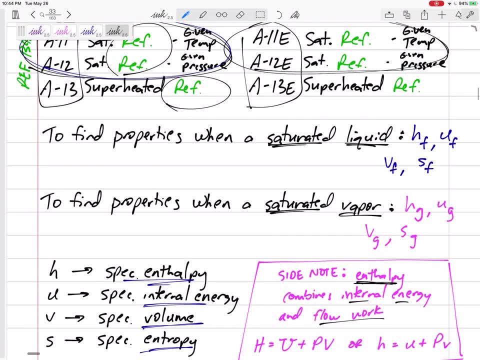 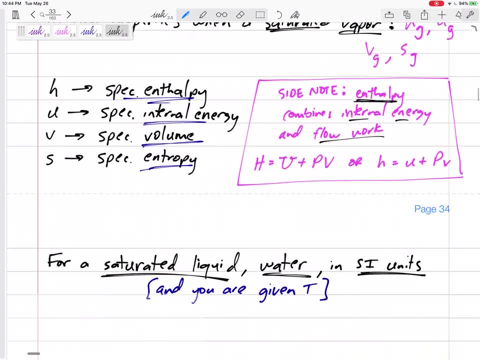 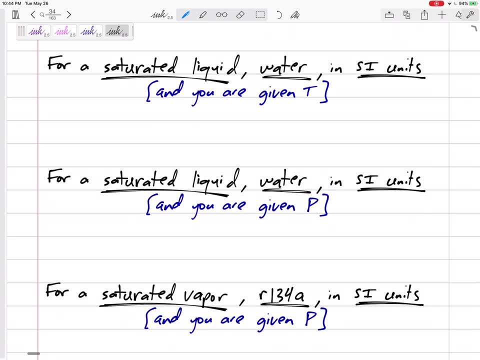 All right. So saturated liquids: we look for the subscript F. Saturated vapor: we look for the subscript G. Let's give an example. All right, So we're going to do lots of examples real quickly. But let's say I have a saturated liquid. 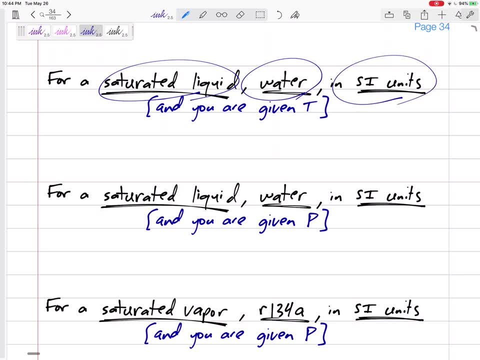 It is water And we're in SI units And I'm given the temperature. Here's the order that I look at. All right, First, I think, SI or English units. All right, So first SI or English units, because SI is appendix one. 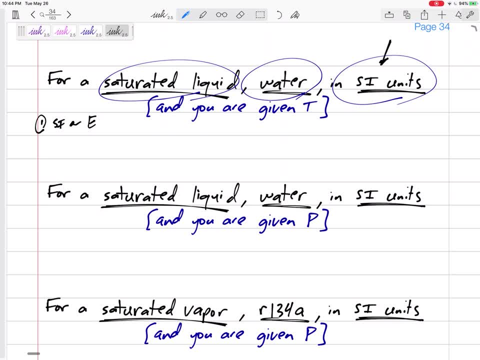 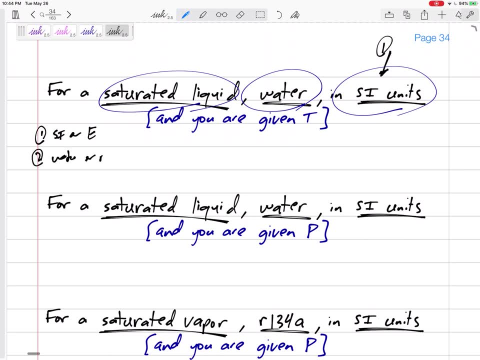 English is appendix two, So SI. So start here. We're in SI units. Then I say water or refrigerant. Okay, Because water our table is four, five, six, seven. Refrigerant table is 11,, 12,, 13.. 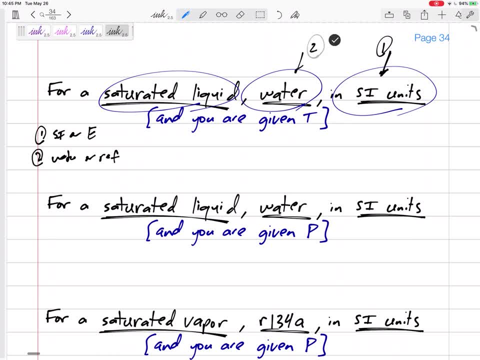 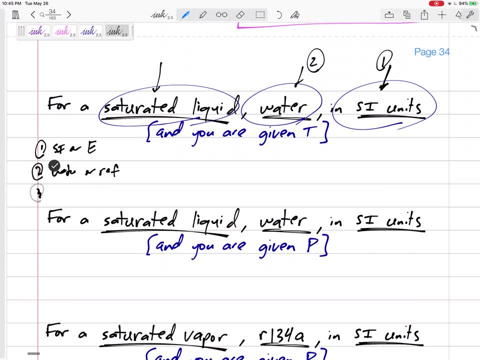 All right, This is water. So I know I'm in four, five, six, seven, And then if it's saturated, saturated or not. So if it is saturated, then I'm in tables four or five, All right, And then I am given temperature. 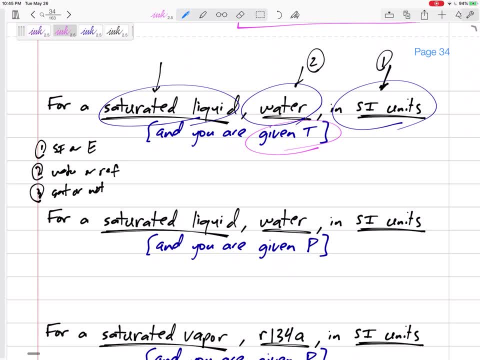 That would be the temperature table, table A4.. So for this one I would be looking at table A4 and I would look for that temperature that I'm given And I would look for subscript F because it is saturated liquid. Okay. 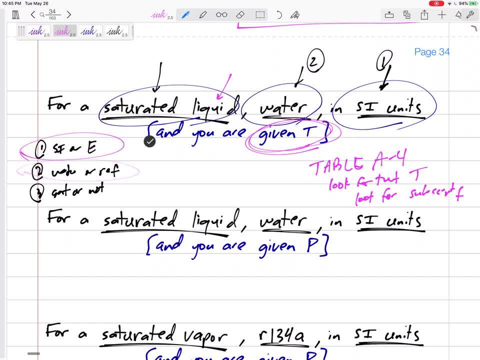 So first SI or English units. Second: is it water or refrigerant? Third: is it saturated? Either saturated liquid, saturated vapor or saturated liquid vapor mixture. So then I would go to tables four or five, If it is superheated. 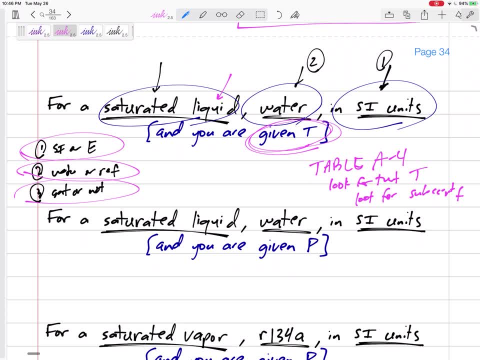 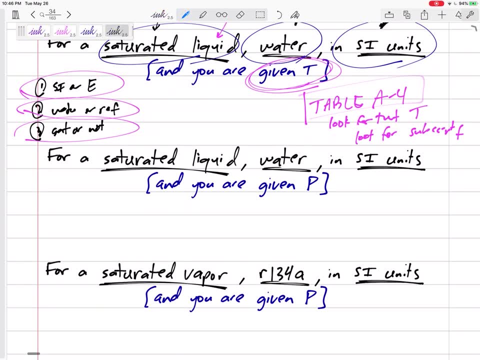 I go to table A6.. If it is compressed liquid, I go to table A7.. All right, But this one is table A4.. All right, How about this next one? Let's try this next one on here. Maybe pause it for a second and say: 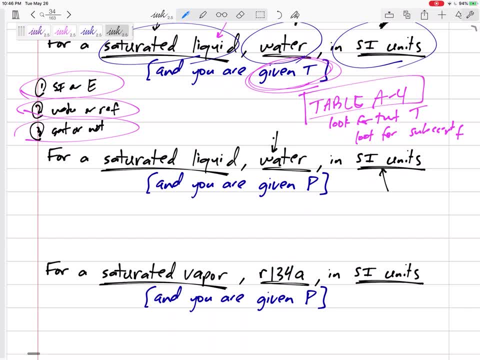 okay, if I have a problem where I'm given SI units of water and it's a saturated liquid but I'm given pressure, what do I look at? So if it's SI units- I know I'm in appendix one- If it's water, 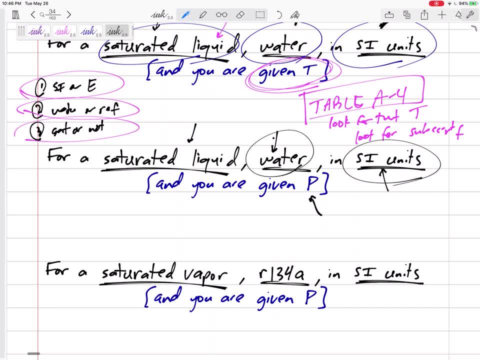 I know I'm tables four, five, six, seven, If it is saturated. I know I'm tables four or five. All right, Which one? Four or five? I'm given pressure. I need to go to the pressure table. 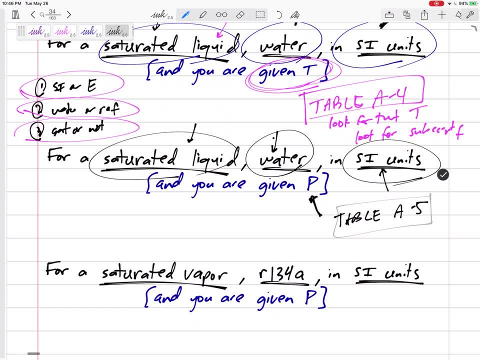 table A5. And I would take that pressure and look for the subscript F for saturated liquid. We'll do a lot of these problems but I want us to just kind of. this is our process: First SI or English units, then water or refrigerant. 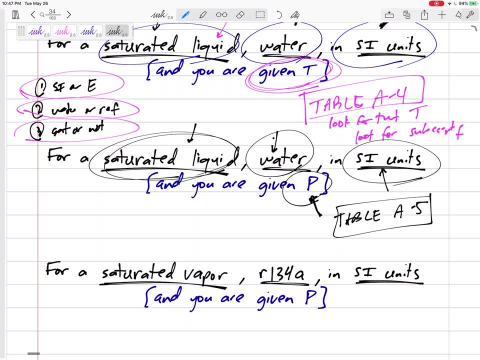 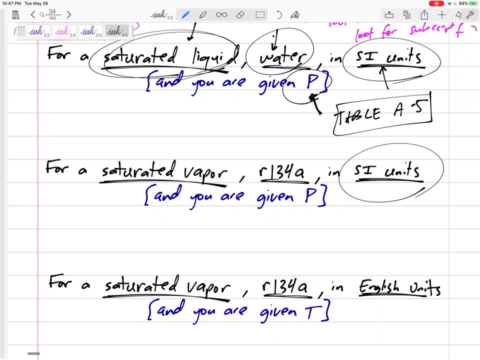 then saturated or not, and then pressure or temperature. All right, How about this next one? We're in SI units, so appendix one, not the appendix with all those E's on the end of it, not appendix two: Refrigerant. 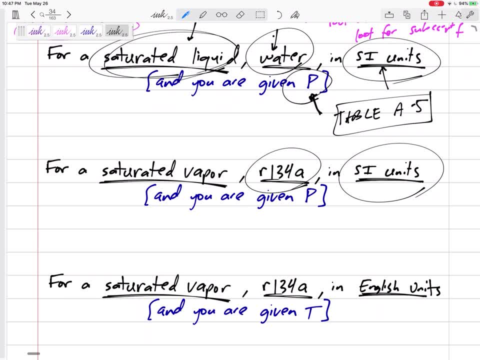 Okay, Refrigerant, I'm looking at tables either 11,, 12, 13.. All right, 11,, 12, or 13.. Saturated, so I'm looking at tables 11 or 12.. And then I'm given P. 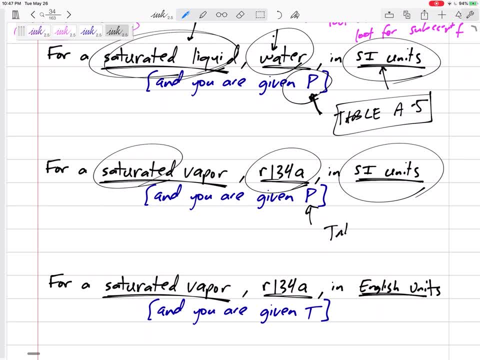 so I'm looking at table 12. Table A12. And it's a vapor. so I'm going to look for subscript G. at that pressure, At that pressure. All right, One last one, then we'll do some problems. One last one. 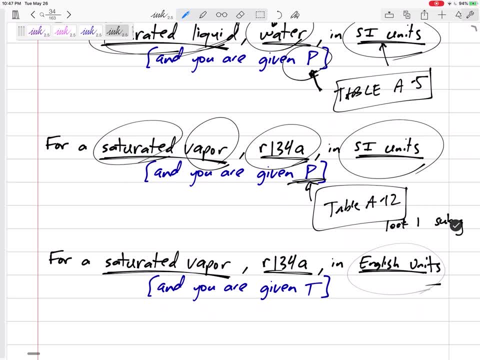 Okay, I'm in English units, so I'm in appendix two. You know appendix with all those E's on the end. I'm in appendix two, Refrigerant. So I'm looking at 11,, 12, or 13E. 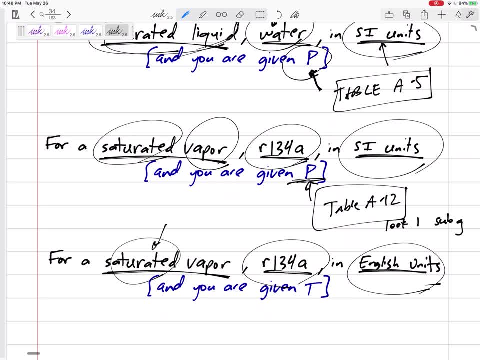 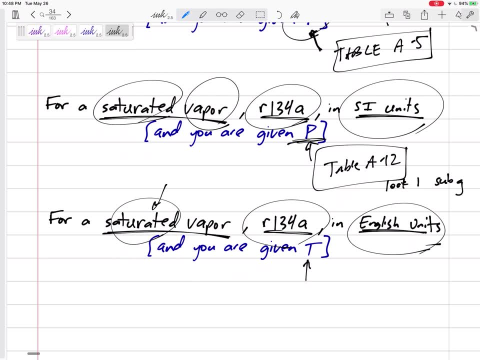 All right, 11E, 12E, 13E. It is saturated, so I'm looking at 11 or 12E, All right, And we're given the temperature, so I'm looking at the temperature table A11E.